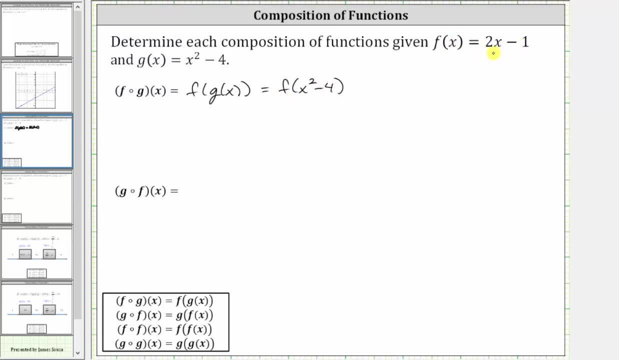 and since f of x is equal to two x minus one, we substitute x squared minus four for x, which gives us two times the quantity x squared minus four minus one. and now we clear the parentheses by distributing and then combine like terms: 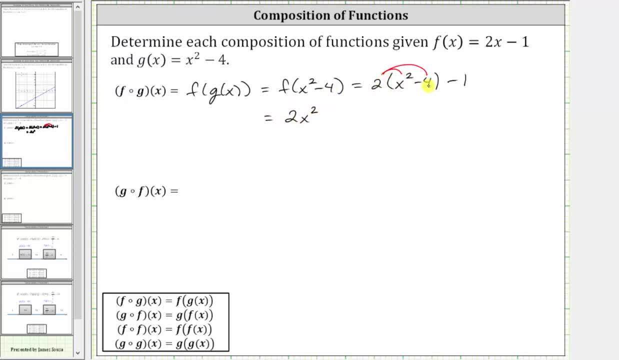 Two times x squared is two x squared. two times negative four is negative eight, giving us minus eight and then minus one, which simplifies to two x squared minus nine. F of g of x is equal to two x squared minus nine. 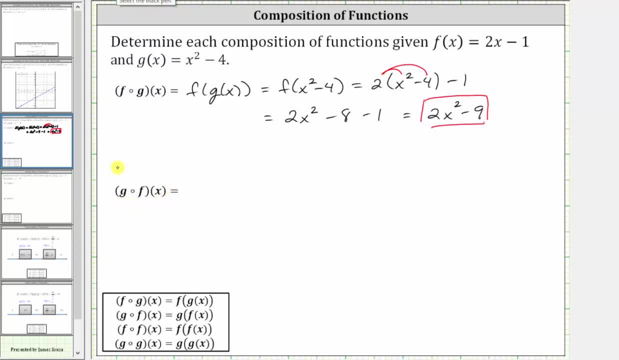 Next, we have g of f of x, which we write using the alternate form, which is still g of f of x, but in a different form Again, because we don't have a numerical value to sub into the inner function f of x. 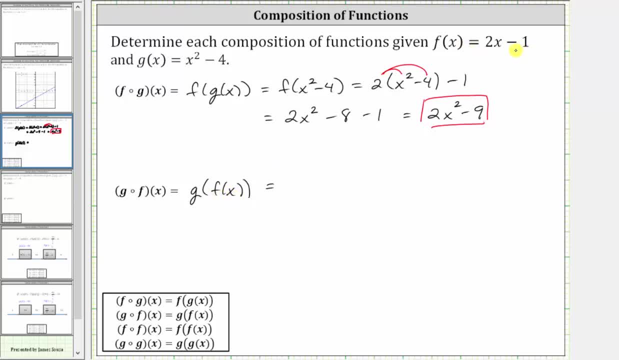 we substitute the function rule for f of x, which is two x minus one, which gives us g of the quantity two x minus one, and now the function rule for f of x becomes the input into g of x, and since g of x equals x squared minus four, 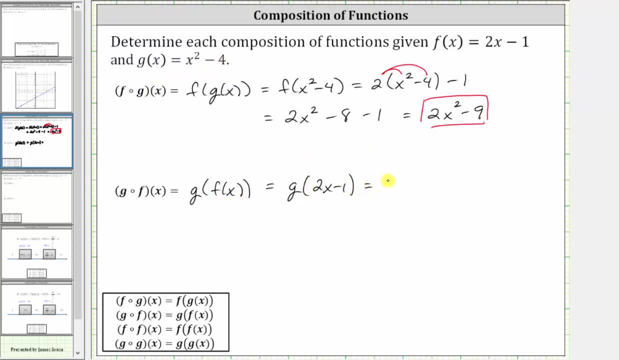 we substitute two x minus one for x, which gives us the square of two x minus one and then minus four. Now we need to multiply this out and combine like terms. To multiply it out, we write out two factors of two x minus one. 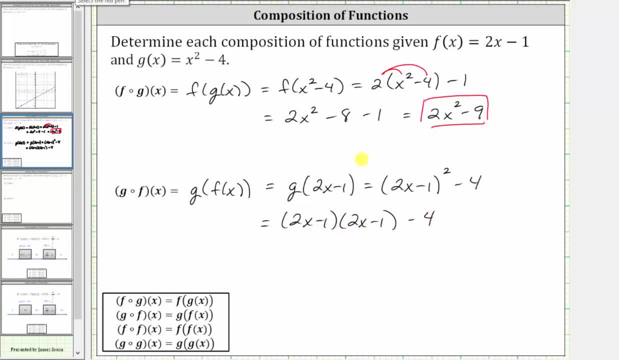 and multiply and then subtract four To multiply two binomials, we have four products: one, two, three, four, two x times two, x is four x squared. and then we have two x times negative one, which is negative two x. 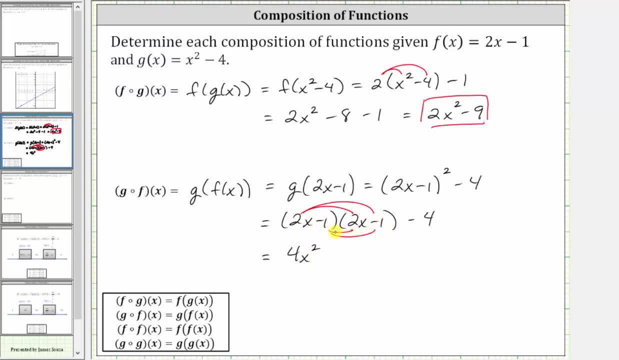 The next product is negative one times two x, which is also negative. two x, Negative two x plus negative two x is negative four x, giving us minus four x, and then negative one times negative. one is positive one, giving us plus one, and then we have minus four. 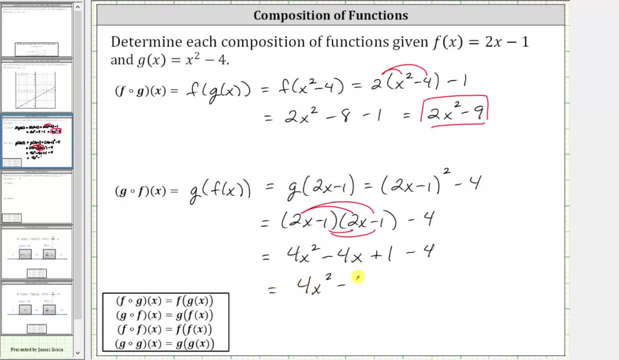 Combining like terms, we have four x squared minus four x, and one minus four is negative three, giving us minus three. G of f of x is equal to four x squared minus four x minus three. I hope you found this helpful.